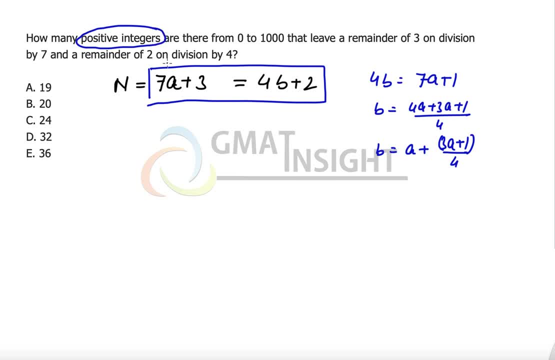 because we are looking at only the positive integer. So since a is an integer, 3a plus 1 should be divisible by 4.. Now, for what values of 3a plus 1, it will be divisible by 4 for failures of f. 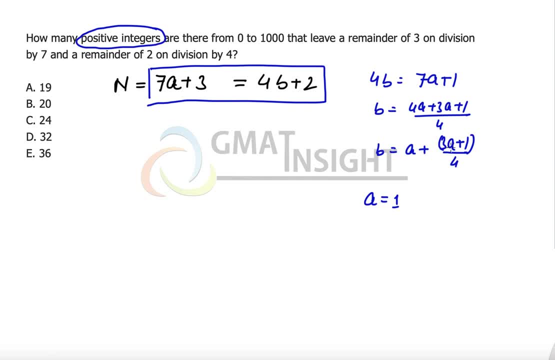 So we can see that the first value of a is equal to 1, because if you substitute a equal to 1, 3 into 1 is 3 plus 1 becomes 4 and 4 is divisible by 4.. And for a equal to 1, the 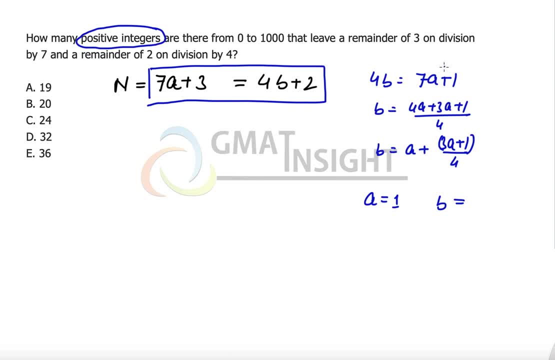 value of b becomes equal to. we can simply substitute the value of a here. So that is 8 divided by 4, b is equal to 2.. Now there is one rule. if you see my concept videos, you will be able to see in that- that in any such equation, when we have to find out the 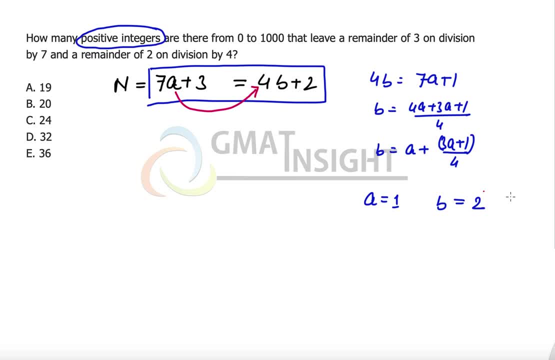 solutions. the value of a always differs from the value of b, So we can simply substitute that and then we can verify that the value of a always differs by the coefficient of b And the value of b always differs by the coefficient of a. By that I mean that the 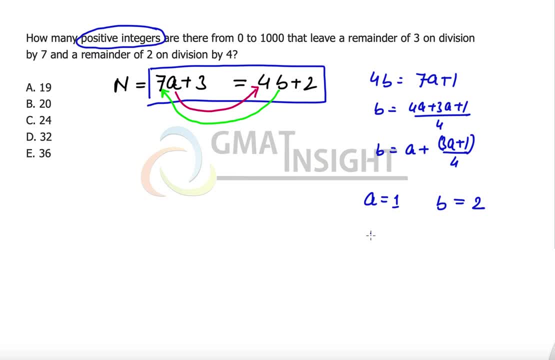 values of a will next be differ by 4,. that means the next value of a will be 5,, 4 greater than 1, right, And in that case the next value of b will be changing by 7,. that means: 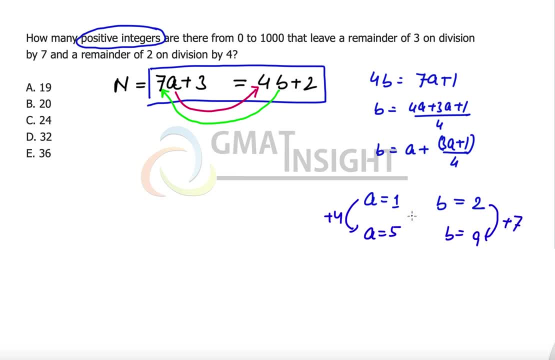 7 plus 2, it becomes 9.. We can substitute that as well, and then we can verify it. So, if you want, for example, if we substitute a equal to 5 here, 5 into 3, 15, 15 plus 1. 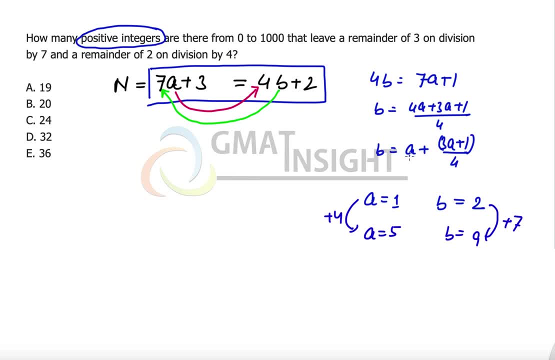 is 16, 16 divided by 4 is 4, and 4 plus 5 is equal to 9.. So that means we can keep getting solution. that means the next value of a will be 9 and the next value of b will be for. 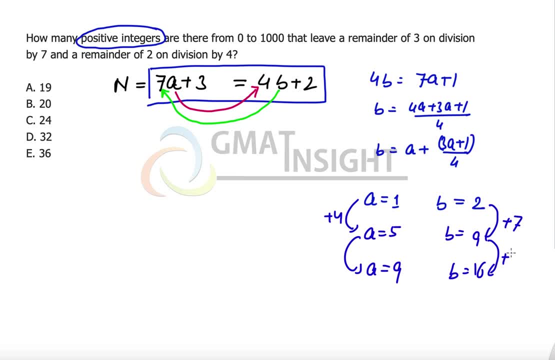 that value of a will be plus 7,, that is, 16.. So these variations will keep giving us the next solutions. Now we have to understand that 7 plus 2 is equal to 9, right. So we have to understand that a plus 3 should be less than or equal to 1000,. all right, And 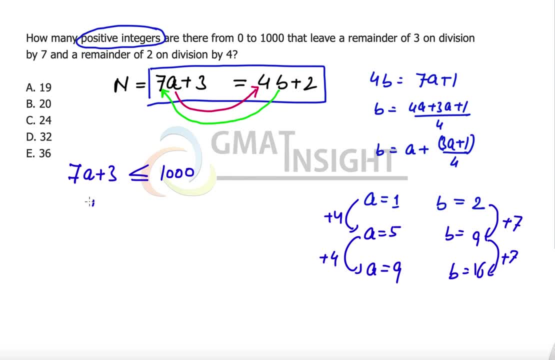 the values of a are getting differed by 4.. So we can simplify this once again: that the value of a should be less than or equal to 1000 minus 7, which is 997 divided by 7.. So we can further simplify this: a has to be less than or equal to 7 minus 7, 7 plus 4. 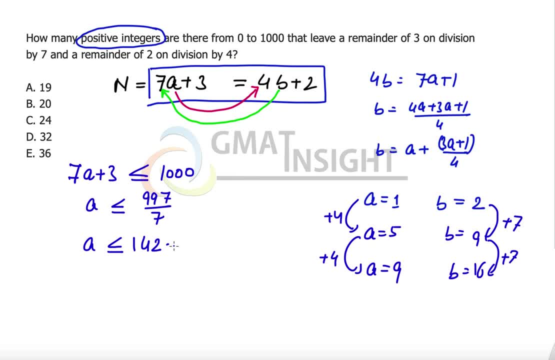 is 28,. 7 plus 2 is 14.. That means the values of a can change from 1 to 142.. So how many values of a will we have in that case? So now for the values of a. we have actually an arithmetic progression. 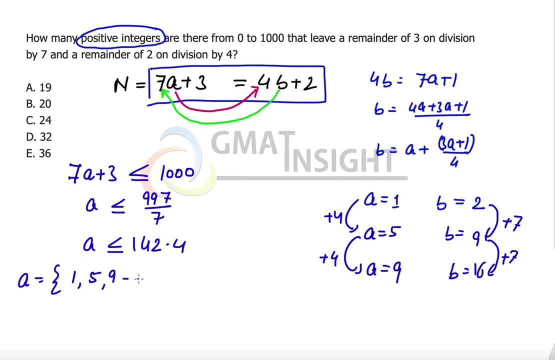 in which the first term is 1,, the second term is 5,, the next term is 9, it keep going on and on. We have to find out the last term. let's call it nth term, and that tn should be less than or equal to 142.. 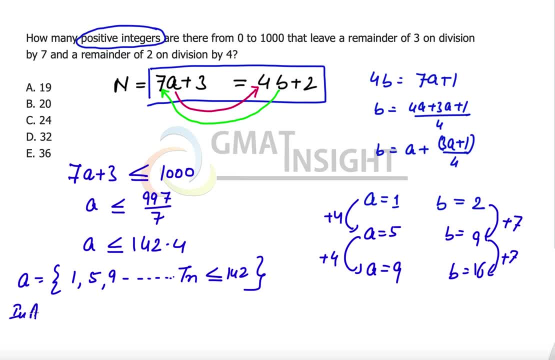 Now, in case of an arithmetic progression. in any arithmetic progression the nth term is defined by a plus n minus 1 multiplied by d, where a represents the first term, d represents the common difference. Here the first term a is 1,. the common difference d. 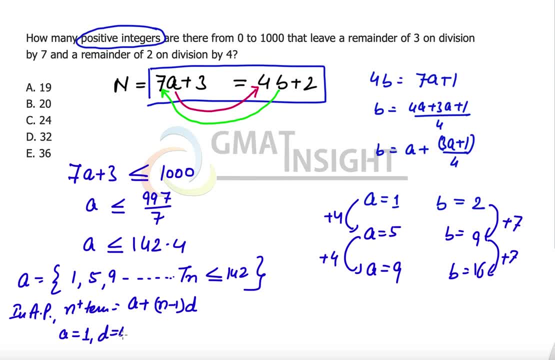 is equal to the difference between any two consecutive values, that is equal to 4, and we will have to find the value of n. So a plus n minus 1 into d should be less than equal to 142, right? so let's quickly simplify this: the value of a. let's substitute 1. 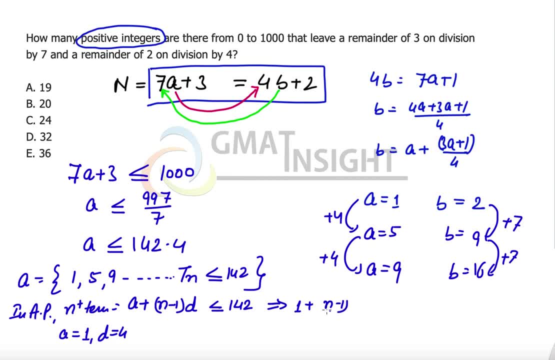 so 1 plus n minus 1 multiplied by 4 should be less than equal to 142. that means n minus 1 should be less than equal to 141 divided by 4, which also gives us that n minus 1 should be less than or equal to 4. 3 times 12, 2 left and 5, that means the value of n. 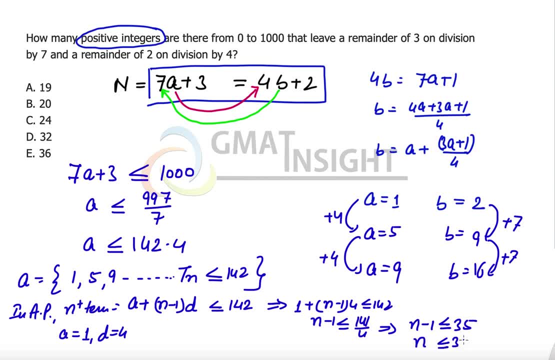 should be less than or equal to 36. now the maximum value of n that are possible are 36. that means there are 36 such possible values and hence we will have 36 solutions. so the answer to the question becomes option e. so it's a very good question to understand.